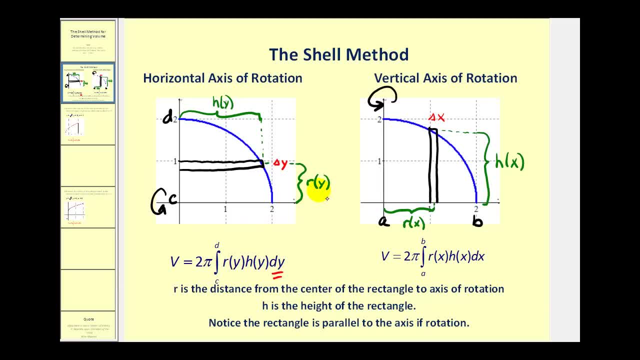 rotation will be the radius or r of y, And the height of the rectangle will be h of y. Again, both must be expressed in terms of y. And then, lastly, because we're integrating with respects to y, the limits of integration from c to d will be along. 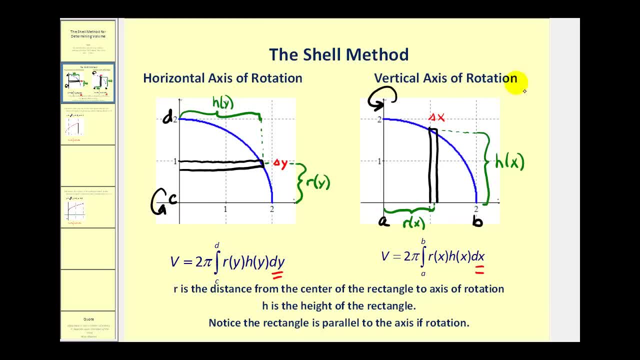 the y-axis And for a vertical axis of rotation, the rectangle will also be vertical or parallel to the axis of rotation. And since the width of the rectangle is delta x, we integrate with respects to x. So this would be the radius in terms of x and this would be the height in terms. 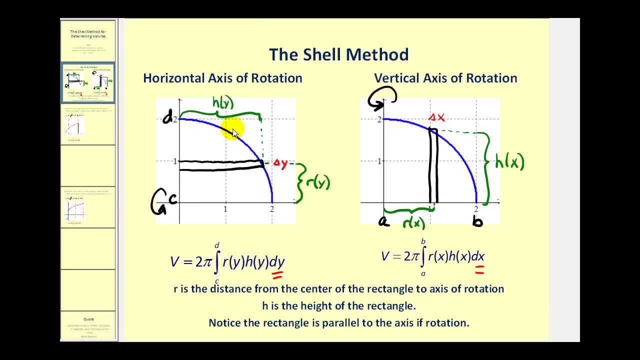 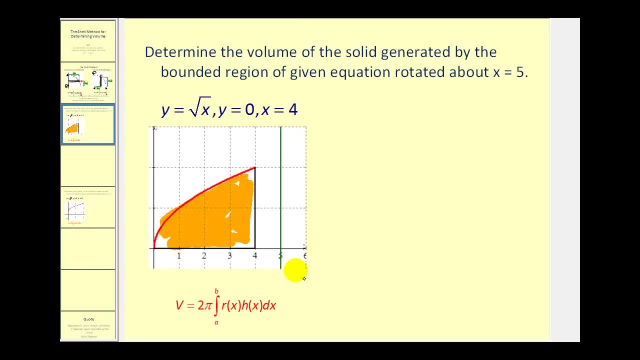 of x. Let's go and take a look at two examples. In this problem we will rotate this region about the vertical line. x equals five. So since we're rotating about a vertical axis, our rectangle will also be vertical or parallel to this. 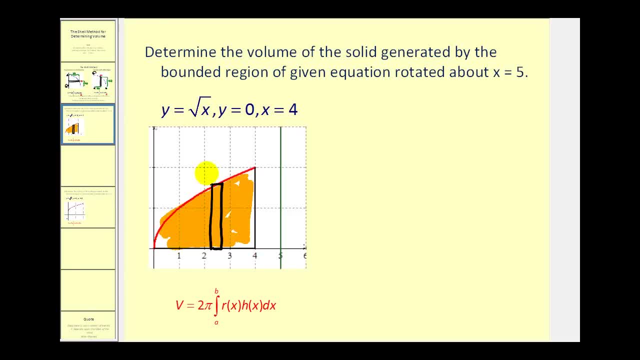 line. So it would look something like this: And since the width of this rectangle would be delta x, we will integrate with respects to x. So let's see if we can set this up using the shell method. The volume is equal to two pi times the definite integral of the. 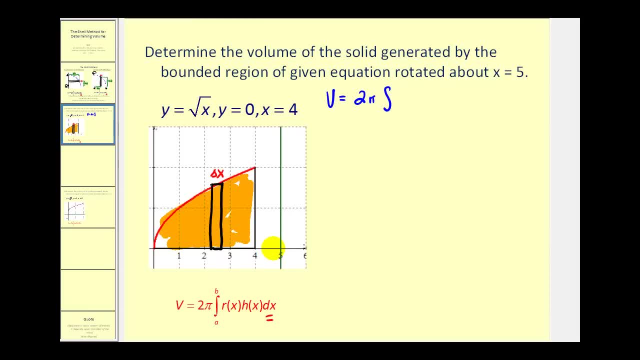 radius times the height. This is going to take a little bit of thought. Well, this distance here would be r of x. We have to think about how we want to express this. It's determined by the distance from the red function to the green vertical line. 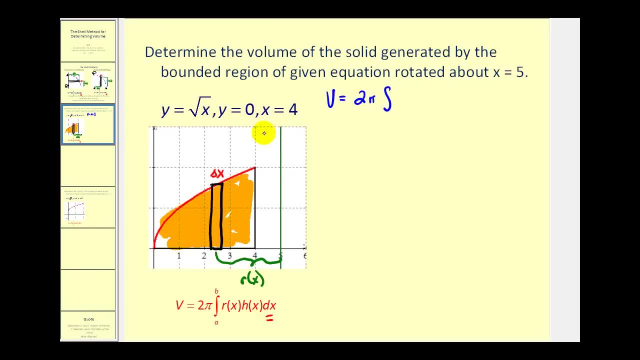 Well, we do know the distance from the y-axis to x equals five, is equal to five units. So if we take five and subtract this distance here, we would have our expression for the radius function And this distance here would be equal to x. So r of x is going to be equal to five minus x. Now we have to. 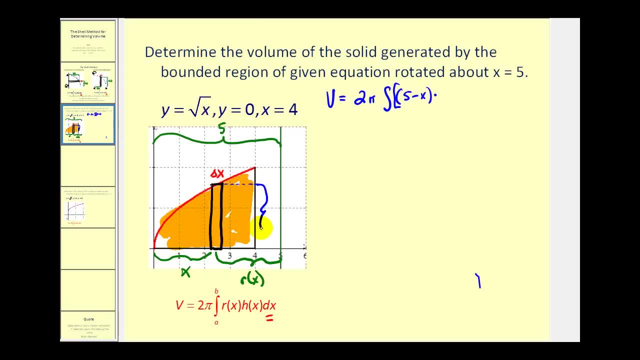 determine the height of this rectangle, and that would be equal to this distance here, And this is equal to y on the given function, and y is equal to the square root of x. So h of x is just going to be the square root of x And since we're integrating with respects, 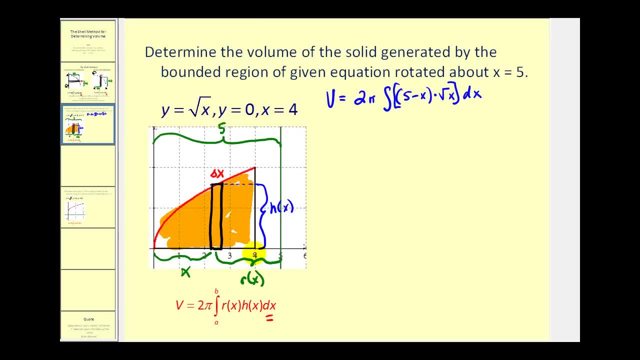 to x, the limits of integration will be from zero to four. Let's go ahead and multiply this out. Remember this is the same as x to the one-half. So we have five x to the one-half Minus this is x to the first times, x to the one-half, That would be x to the three-halves. 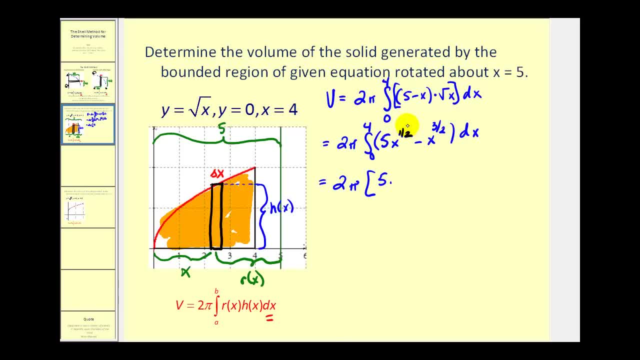 Now we'll go ahead and find the antiderivative. So adding one to one-half, that will be x to the three-halves divided by three-halves Minus three-halves plus one would be five-halves. 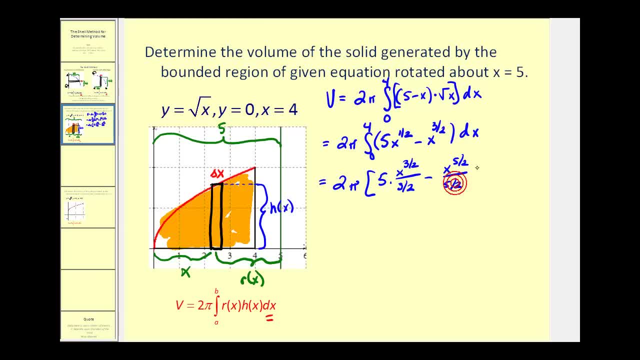 So x to the five-halves divided by five-halves. So let's clean this up and then we'll perform the substitution. So this will be five times two-thirds, That will be ten-thirds. Again, dividing by five-halves is the same as multiplying by two-fifths. 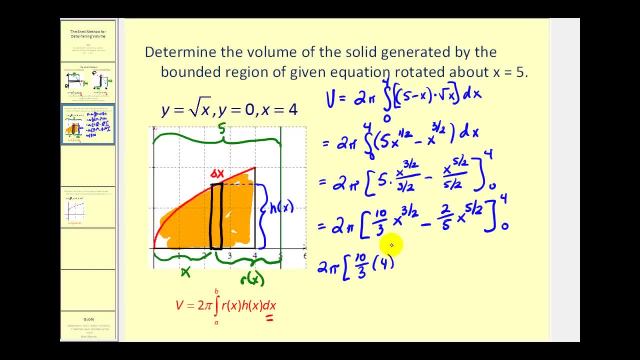 Now we'll replace x with four. We have to take all of this and subtract when x equals zero, but luckily, when x is zero, both of these terms would be zero. To save some time, I've already worked this out- It comes out to 416 pi. 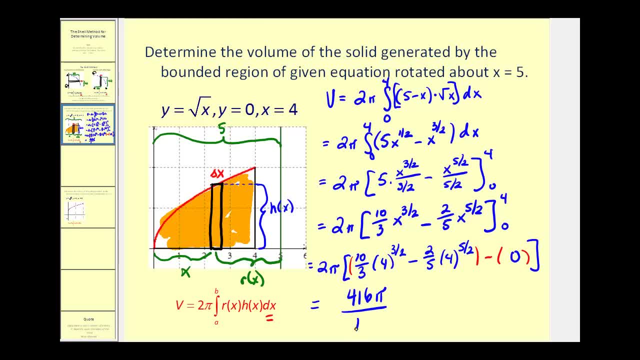 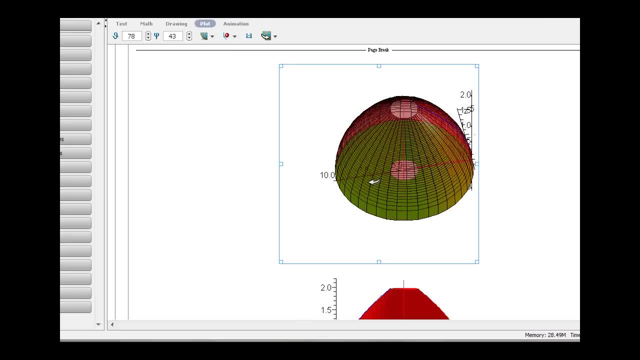 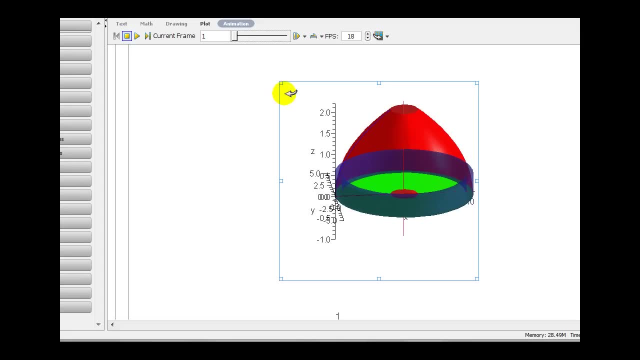 divided by 15, which would be the volume of that solid. It would look like this, And this illustrates what we did: using the shell method, We accumulated the volume of shells as the number of shells approached infinity, which gave us the actual volume of the solid. 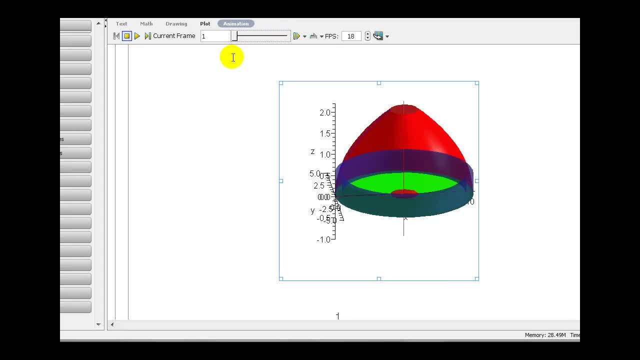 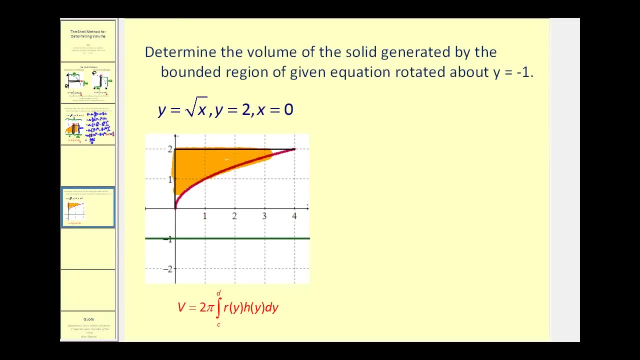 Let's go and take a look at another one. So this would be the bounded region, and we're going to rotate about the line y equals negative one. Therefore, our rectangle is going to be parallel to this horizontal axis. So it might look something like this: And since now the thickness is equal to delta y, 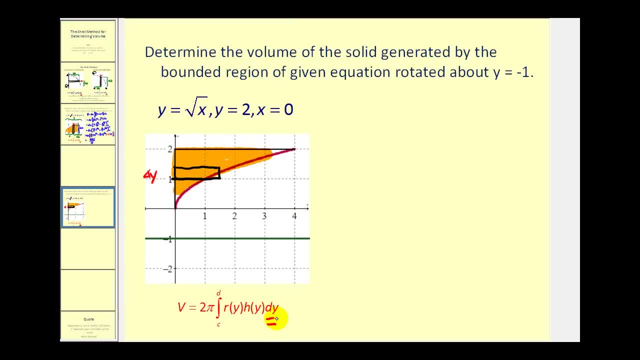 we have to integrate with respects to y. So that's the number of shells that approached infinity, which gave us the actual volume of the solid. So the volume will equal two pi times the definite integral of r of y times h of y. Well, r of y would be the distance from the center of this rectangle. 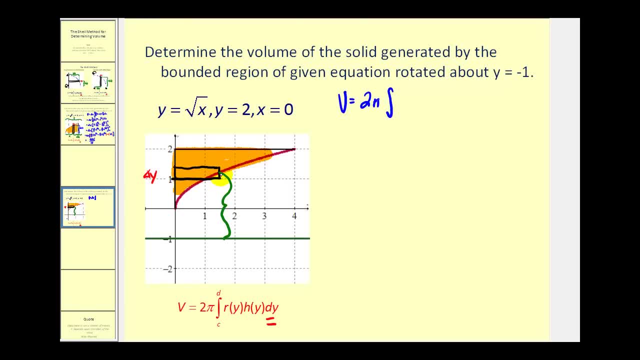 to the axis of rotation. Well, the distance from the function to the x-axis would be y, but we're one more unit away. so this would be y and then plus one. So r of y is equal to y plus one, And the height of the rectangle would be h of y. 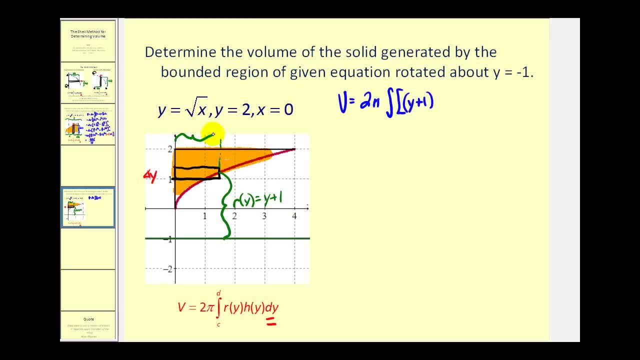 And that would be the distance from here to here. Well, this horizontal distance is equal to x, based upon the function, y equals the square root of x. So we have to take y equals the square root of x and solve it for x. So if we were to take this and square both sides, 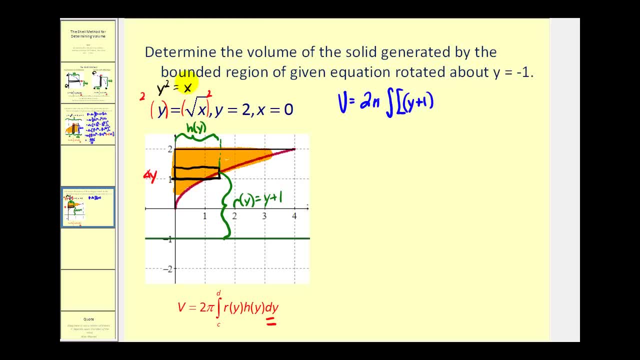 we would have: y squared equals x And that will be the function for the height h of y is equal to y squared. And, lastly, we have to determine our limits of integration, Because we're integrating with respects to y. our limits of integration will be along the 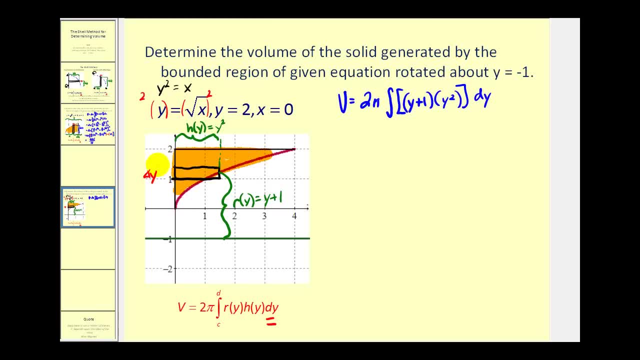 y-axis, So the limits of integration will be from zero to two. Let's go ahead and finish this Now. we'll just distribute the y squared, So we'll have y cubed plus y squared. Now we'll find the antiderivative. 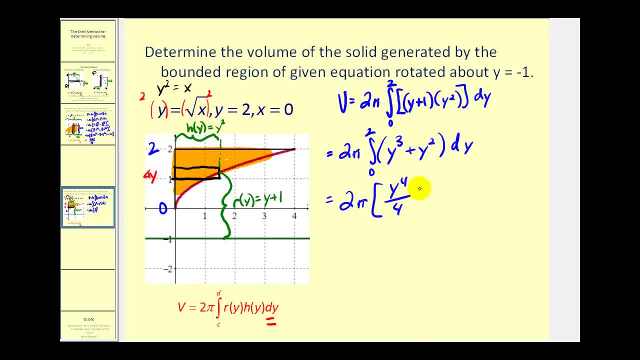 So we'll have y to the fourth over four, plus y cubed over three. Now we'll replace y with two, So we'll have two to the fourth plus two to the third over three, And then, when y is zero, both of those terms would be zero. 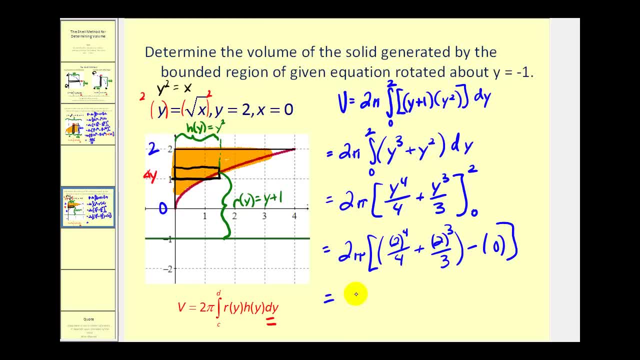 And to save some time, we've already determined this value: It's going to be twenty-thirds. So we have two pi times twenty-thirds, which is equal to forty pi over three, which would be the volume of the solid formed by rotating this region about the line. 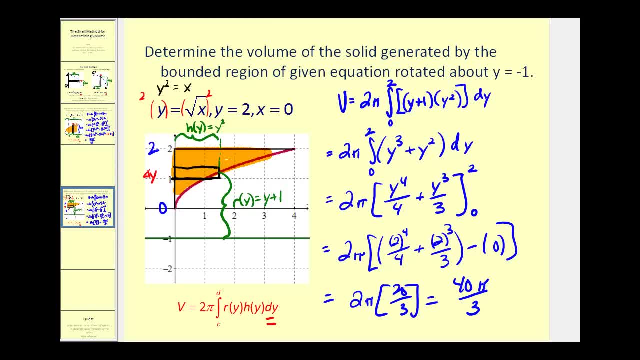 y equals negative one, And that'll do it for now. That'll do it for this video. Thank you for watching.